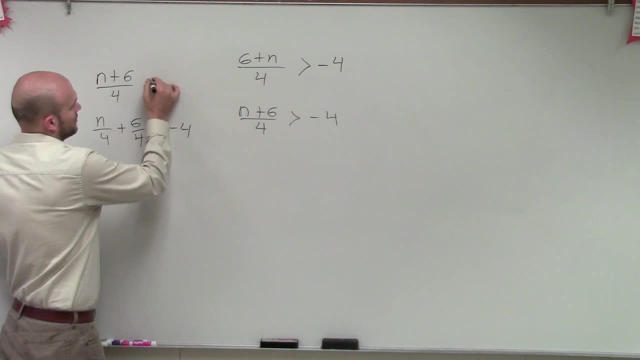 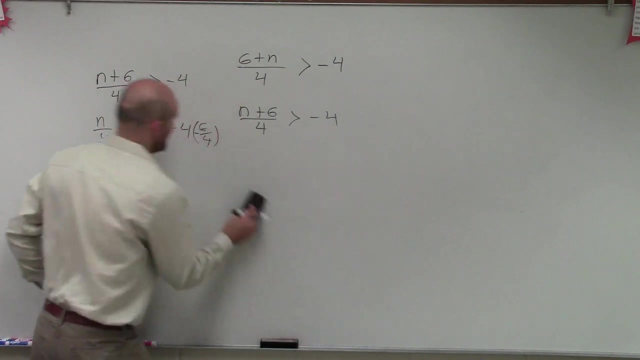 to add something. if I'm going to undo addition, I'm going to have to subtract 6 fourths. Now you can do this. However, we don't really like subtracting. I mean, that's a multiplication. We don't really want to subtract a whole number minus. 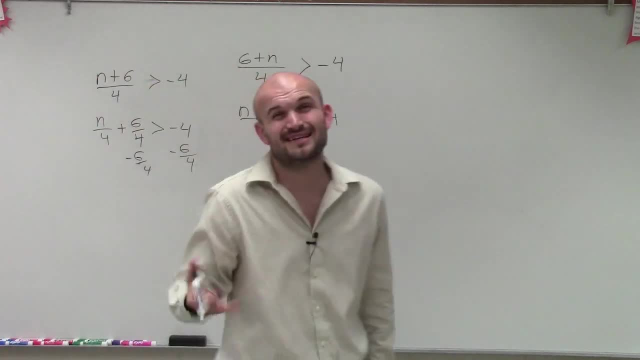 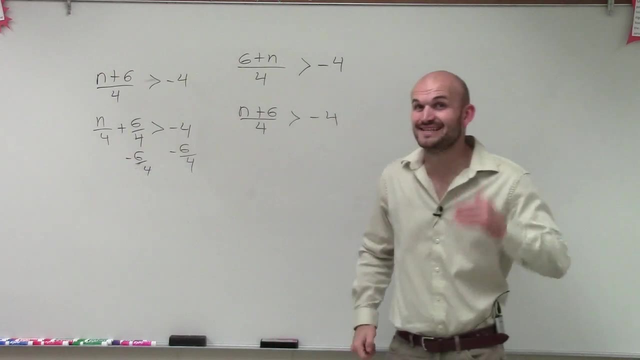 a fraction, because a lot of us have trouble with some fractions And it's just a little bit extra work, right? So what we can do is, rather than having to subtract 6 fourths on both sides, let's just get rid of the fraction, right? I mean, why deal with all that extra? 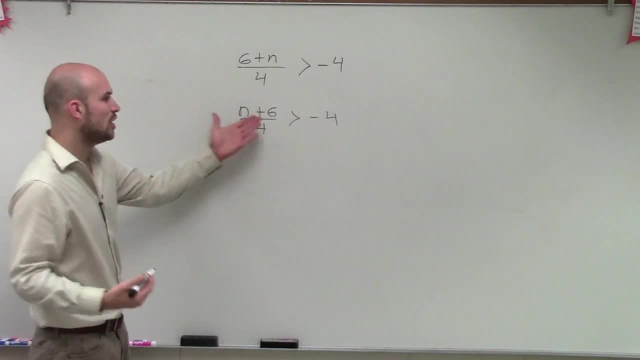 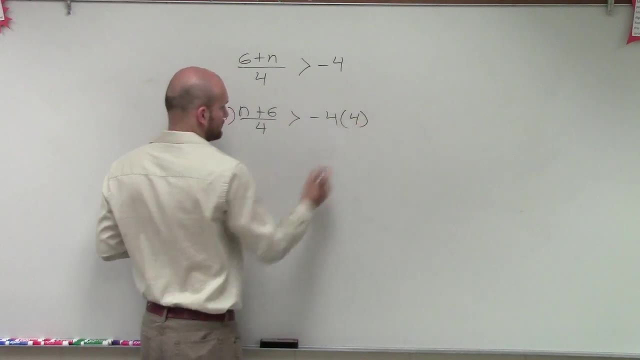 work. So what we're going to do to get rid of the fraction is we're going to multiply by c. So to get this fraction, this means we're dividing by 4. So we're going to multiply by 4. That divides out, because you're multiplying by 4 times a whole expression. So those divide. 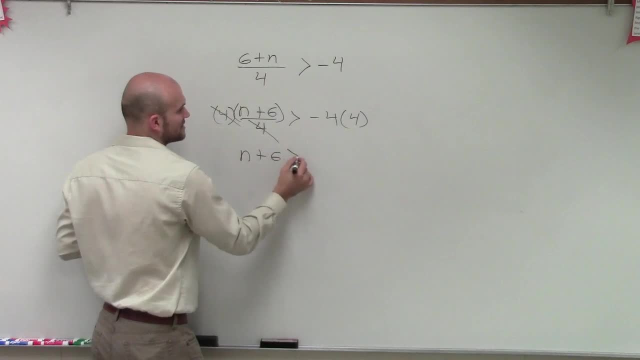 out to 1.. And then we'll get this. So we'll have x, n plus 6 is greater than negative 16.. Now I don't have any fractions and it's very easy for me to use my inverse operations. I subtract 6, subtract 6, n is greater than negative 22. So it means all numbers that. 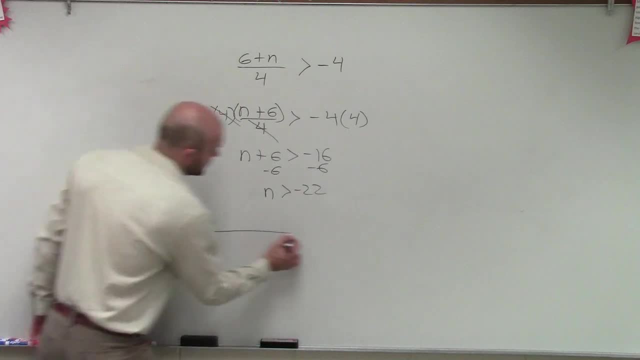 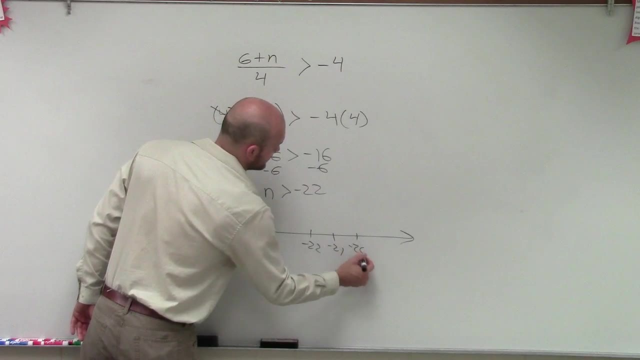 are greater than negative 22.. So I need to represent that now with a number line. All right, so I'm going to start at negative 22. And to the right are going to be my numbers that are less than negative 22. And to the left will be numbers that are less than negative. 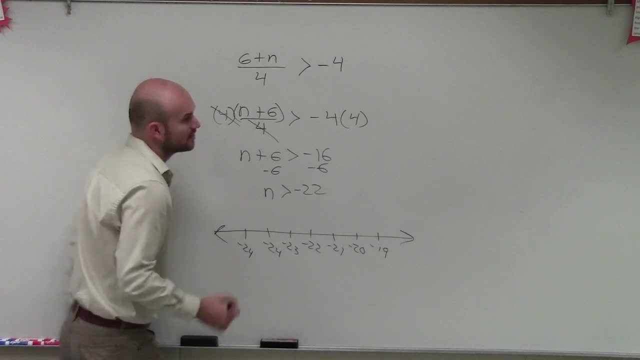 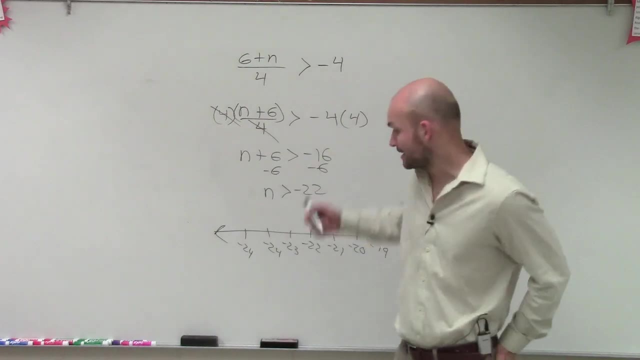 22. And you can just think of less than and greater than, with negative numbers. as far as money, right, If you have a negative amount of money, that means you owe somebody money. So when you owe somebody more in monetary value, then you actually have less. So that's. 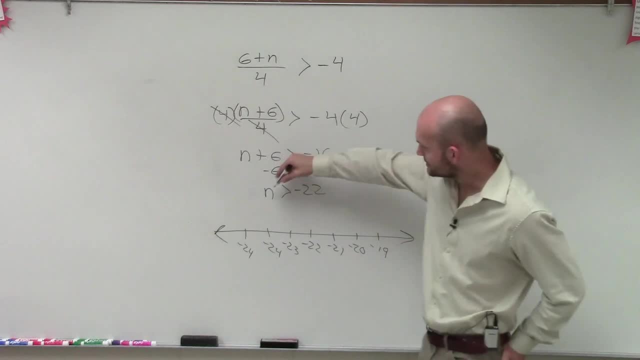 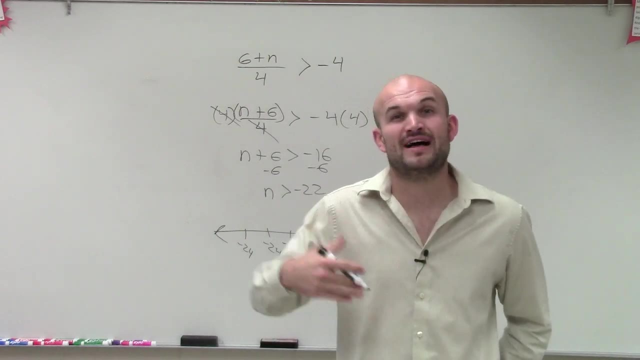 why these numbers are less than negative 22.. So I always start at where my initial value is. Is that negative 22?? Speaker 1: We're going to shade that in if our value equals negative 22. But when I say n is greater than negative 22,. 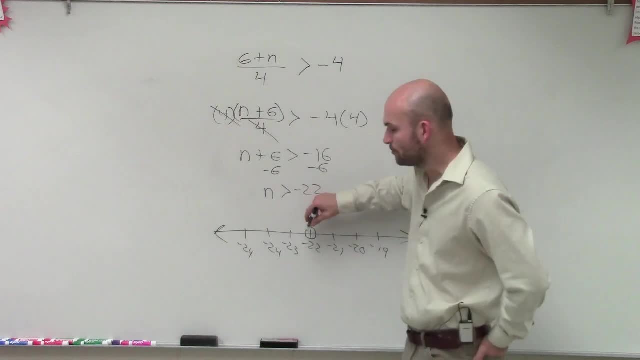 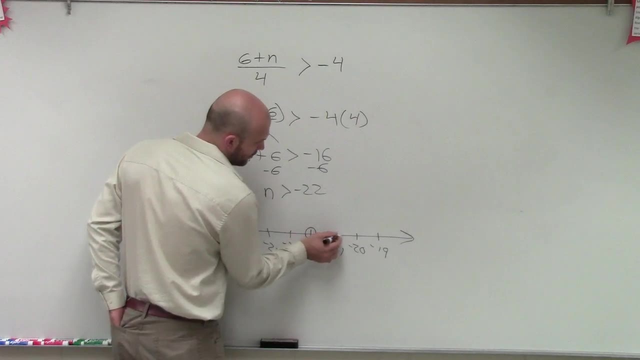 that does not mean n is equal to negative 22.. So therefore that's going to remain open. But then I say: what are the values? So n is greater than negative 2.. What numbers are greater than negative 2?? Well, that's going to be all these points that